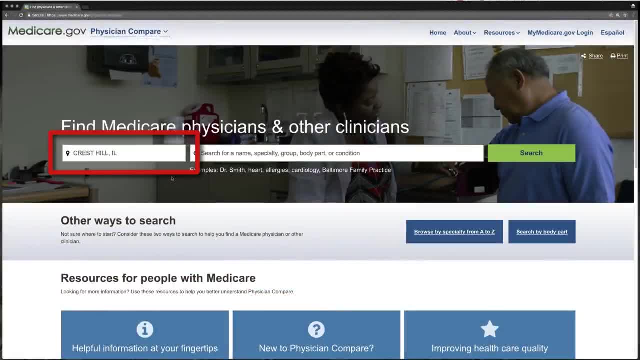 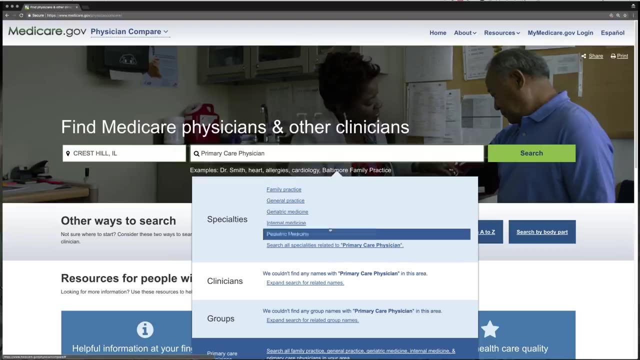 She lives in Crest Hill Illinois. The location box automatically recognizes the location of her computer and Crest Hill Illinois is filled in for her. Linda enters primary care physician into the main search bar. The drop-down box gives a few options for what she may be searching for. 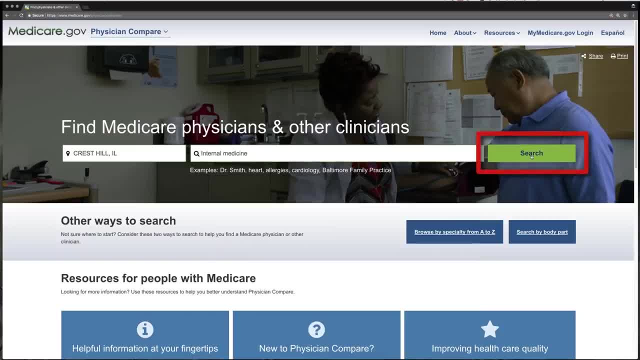 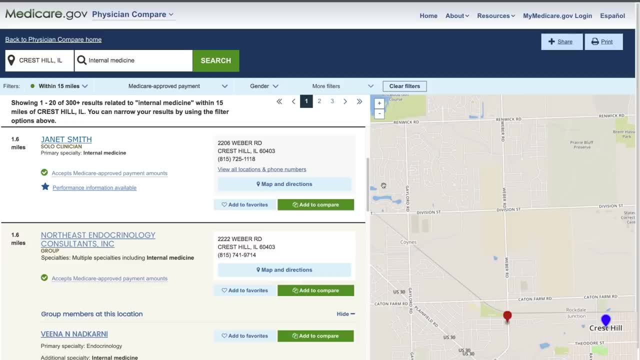 She makes a choice from the drop-down box based on her needs. Here is the results page of physicians who practice internal medicine in Linda's area. Physicians are listed on the left of the page in order of distance. She can pick from either a group or an individual clinician. 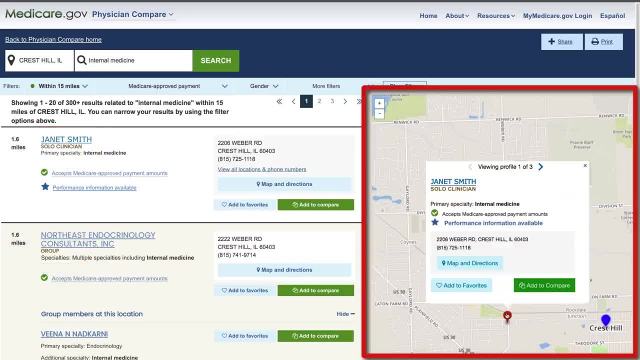 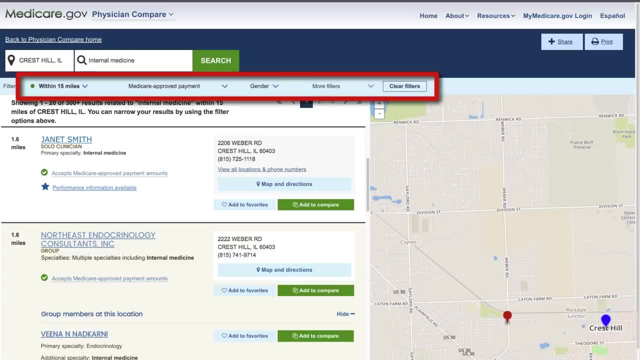 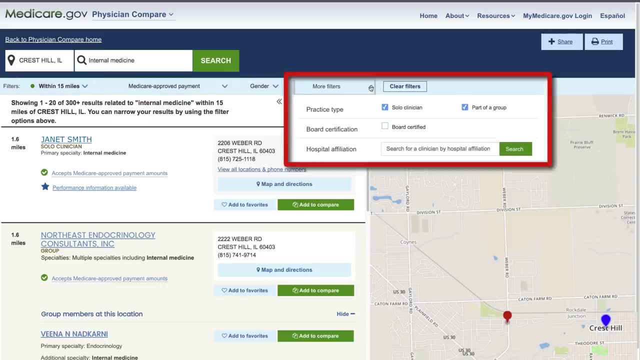 The map on the right has pins to show practice locations. Linda's current location is shown with a blue pin. Linda can use the filters across the top of the screen to refine this list of physicians based on distance, Medicare-approved payment amount, gender and more. 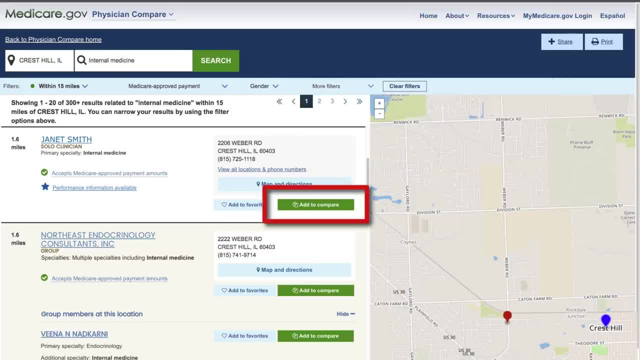 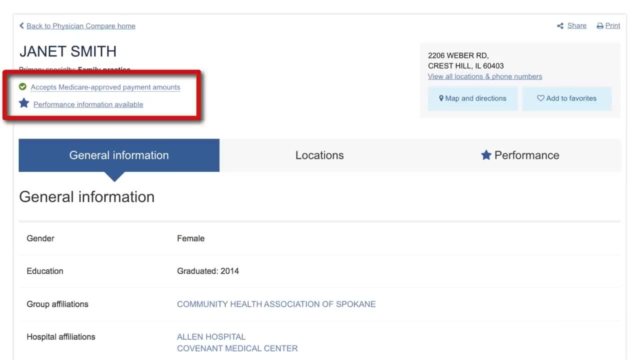 She can use the Add to Compare button on the top of the screen. She can also use the Compare button on a listing to compare as many as three different physicians or three different groups. These two icons indicate that this physician accepts the Medicare-approved payment amount and has performance information available to view. 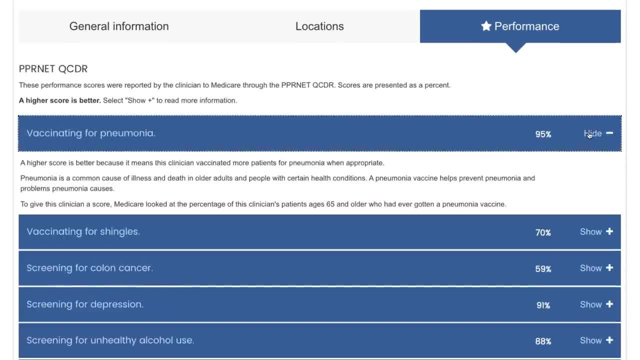 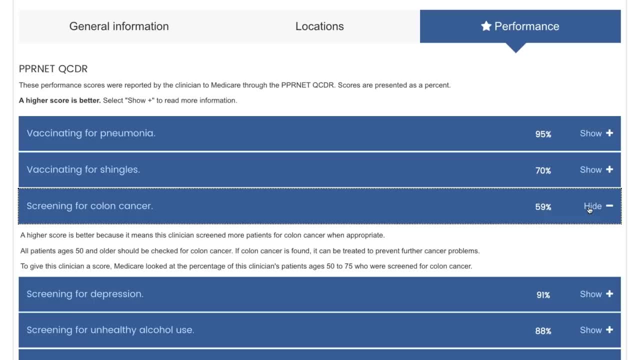 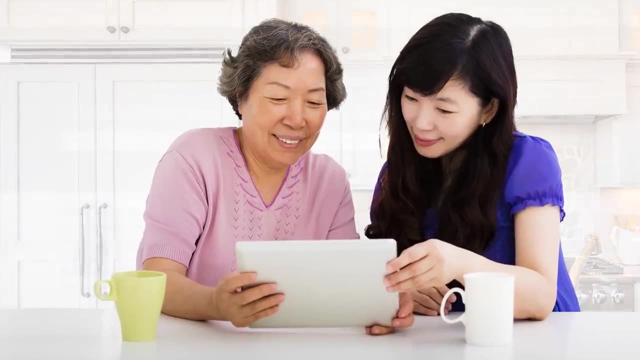 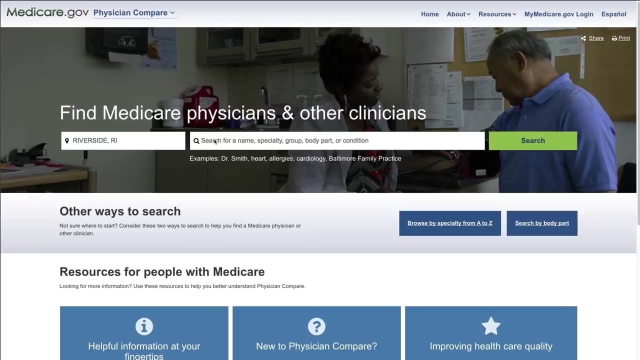 Performance information shows whether the doctor provided patients the recommended care. Now let's see how Mary uses physicians. Mary uses Physician Compare. Mary's current neurologist wants her to get a second opinion for her constant migraines. Mary and her caregiver, Nancy, visit the Physician Compare website and begin their search for a clinician. 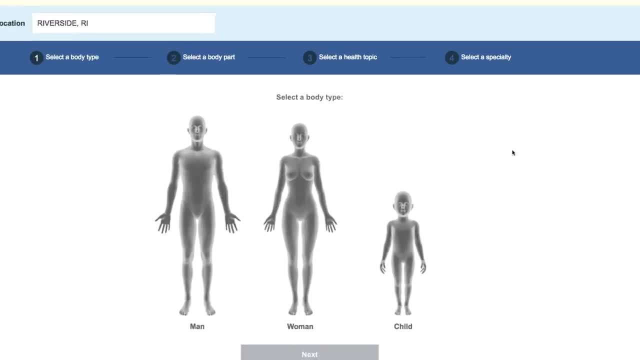 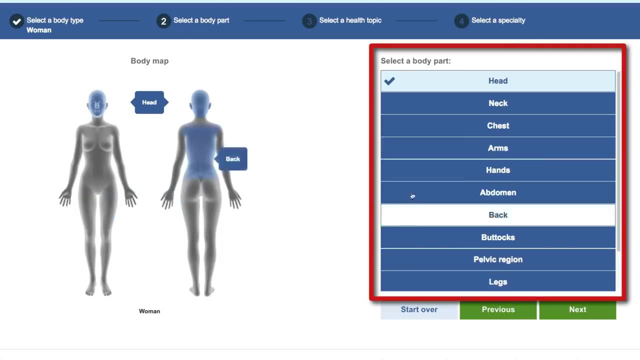 They find the Search by Body Part button. Mary clicks on the diagram of a woman's body. They can pick the area of the body they're concerned about. Mary chooses Head from the list of available body parts on the right and then selects the Next button. 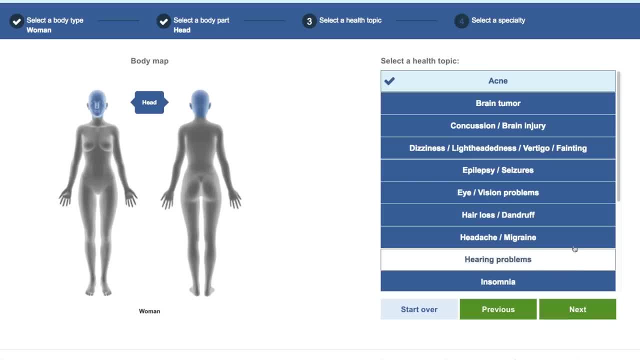 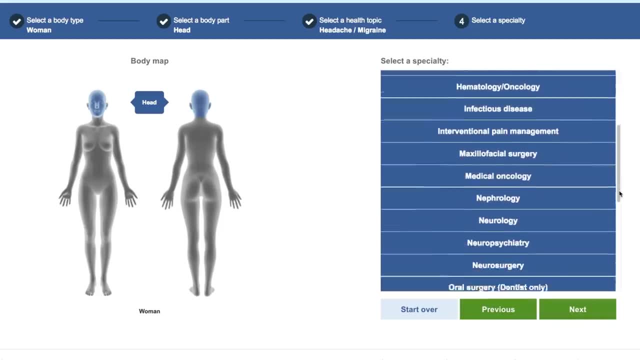 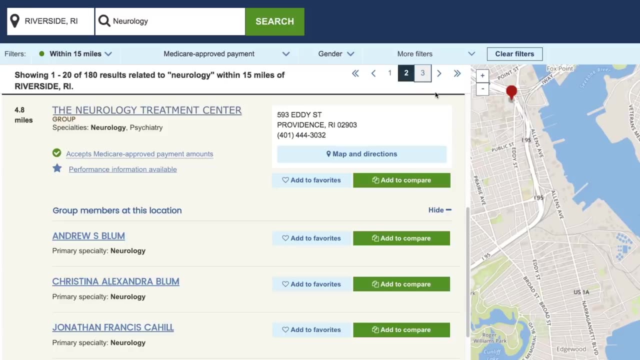 She then selects Headache, slash, Migraine from the list of health topics. She selects Neurology from the list of specialties. Mary is redirected to the results page. She and Nancy select a group from the list. Nancy has a friend who told her she got great care there.